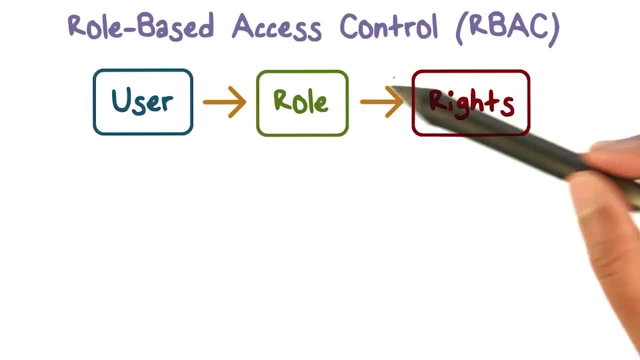 So this part of the policy basically says access rights are defined for roles, And users who are going to log into the system or authenticate themselves to the system can then take on some roles. So, RBAC, the way to think about this is that we don't have direct access. 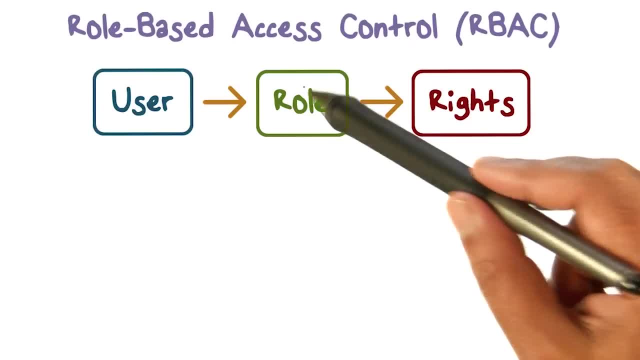 rights for users. Users must be activated into one or more roles And once they assume one or more roles, based on what those roles give them access to, That's what the user or the process running on this behalf of this user can access. 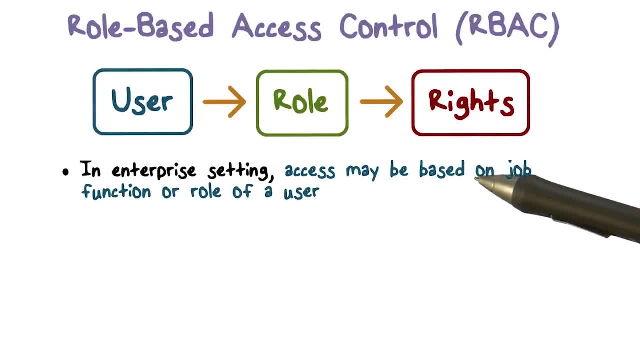 So we're talking enterprise setting. Access may be based on job function or role of a given user. That's where this might make sense. Project manager may have access to all files. Developers or people doing QA or something like that may access files in different ways, and so on. 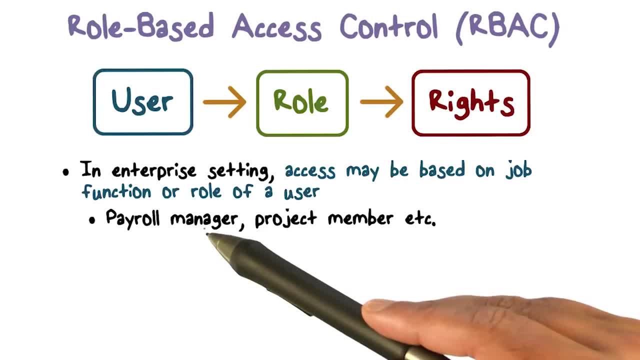 Payroll manager in your HR function may be able to look at files that have people's salaries and so on, because they are Payroll manager and things like that. So this is how roles will be defined: Access rights associated with roles, as we said before. 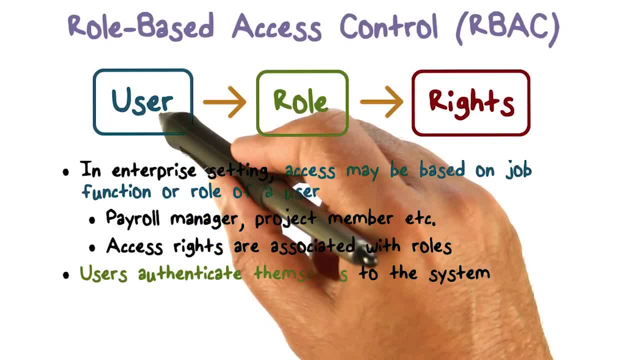 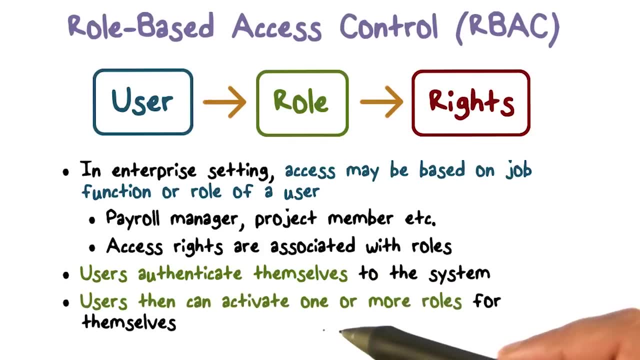 And users and authentication happens and we know who the user is who's logging into the system. We have to then sort of start with authentication but then be able to activate one or more roles for them, okay. So role activation is something else that has to be added to this process. The policy defined here and sort of their. okay, so the policy here and sort of their. the policy defined here and sort of their. okay, so the policy is that you have to and the policy is and they have to be added to this process. 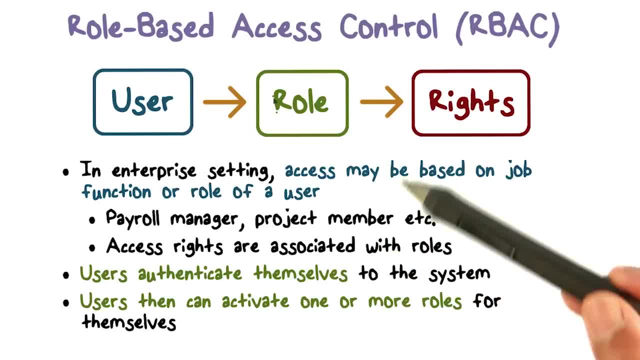 And it's not. they have to be added to this process. So the policy defined here and sort of their role act is that they can't be active, or two stages: activating a role for a user and, based on that, deciding what the user can access. 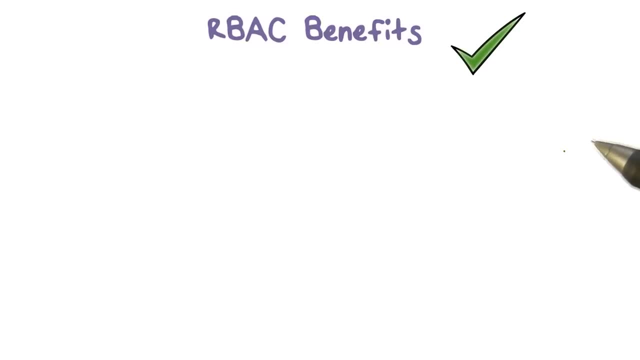 Now there's some benefits that come when we have role based access controls. What could be some of these benefits? So, first of all, we said our policy defines what roles have what kind of access for resources in the system, So the policy doesn't need to change when let's say 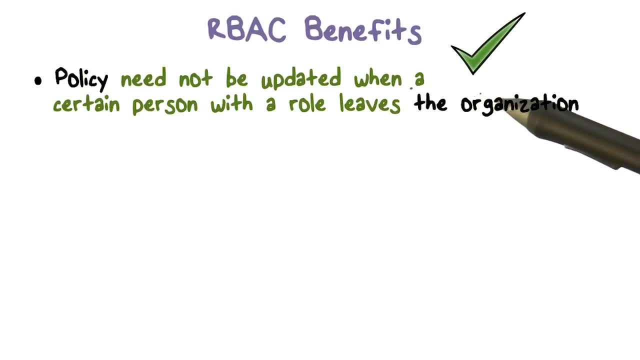 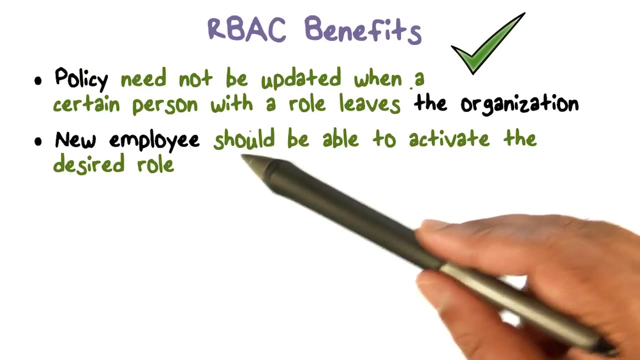 a certain person leaves, the organization Policy is associated with roles. It's not associated with users. So, users coming or going, they don't require changes to the policy the organization has When a new employee comes. basically we think about what role is appropriate for them.